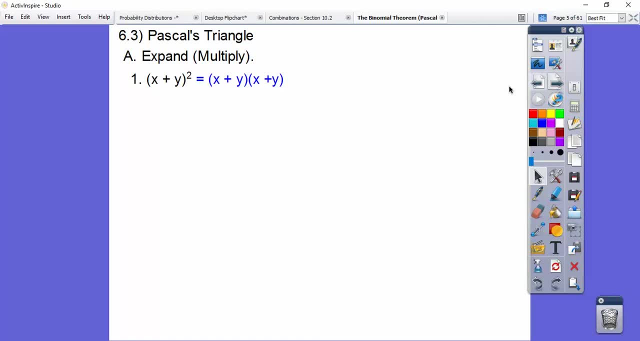 y times x plus y, And if we FOIL it out we'll get x squared And then outer times outer is x- Y, inner times inner is y, x, which is the same as x- y. So we're adding them, So we have. 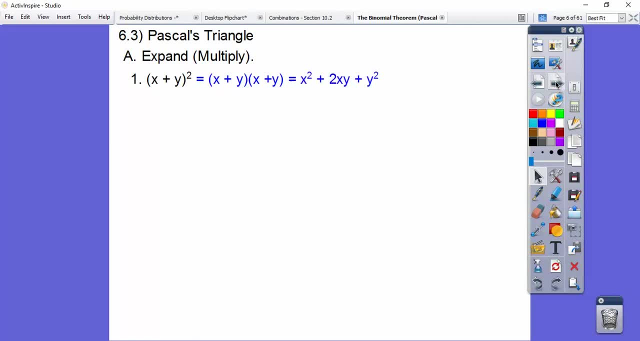 two x y's And then last times last, is y squared. Okay, so x squared plus two x y plus y squared. Okay, So let's expand x plus y cubed. Okay, so well, that's just x plus y times x plus. 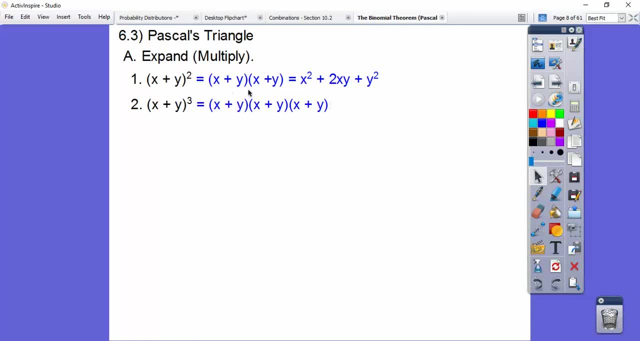 y times x plus y, And then we already know what the x plus y times x plus y is. So I'm going to replace this with this right here, Okay, And then I'm going to distribute the x through and then distribute the y through, So I'll do the x in blue, So, and then we'll 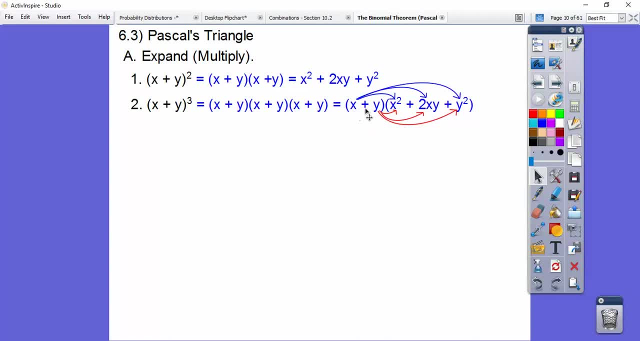 do the y in red. Okay. so x times x squared is x cubed, And then just add an x to everything. So this would be plus two x, x squared, y, and then plus x- y squared. Okay, so that's what. 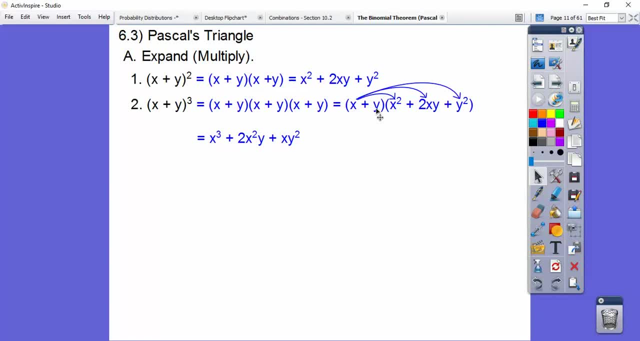 that is All right. and then we'll put the y through. So we're just adding a y with everything. So this is x squared y, And then this will be two x- y squared and then y cubed. Okay, so then when we do that, then we combine like terms. you guys, I have a x, two x squared. 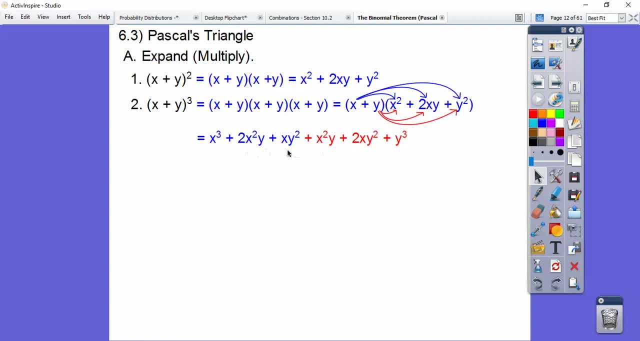 y here, I have another one x squared y here. So we have three x squared y's And, and similarly we have these like terms: x- y squared, and then two x y squared is three x y squared. So there's the final answer right there. Okay. Now, if that wasn't fun, here's x plus y to the fourth: Okay. 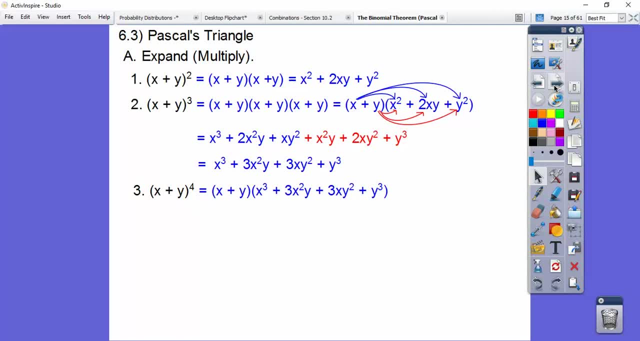 well, that's just x plus y times x plus y, times x plus y times x plus y, And we already know what it's. this answer right here, So we'll do it. So all we got to do is distribute x through again, So. 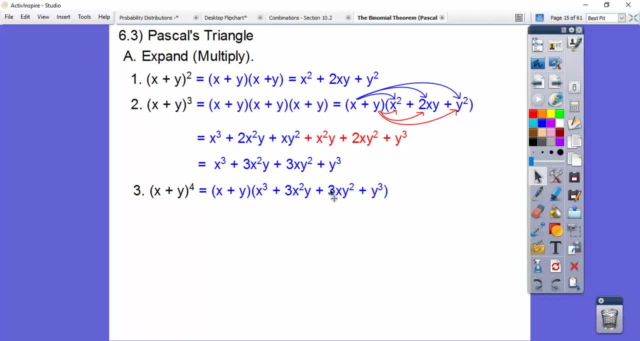 x to the fourth: three x cubed, y, three x squared, y squared, x, y cubed, and then put the y through. so x cubed, y, three x squared, y squared, three x, y cubed, and then y to the fourth. Okay, so there. 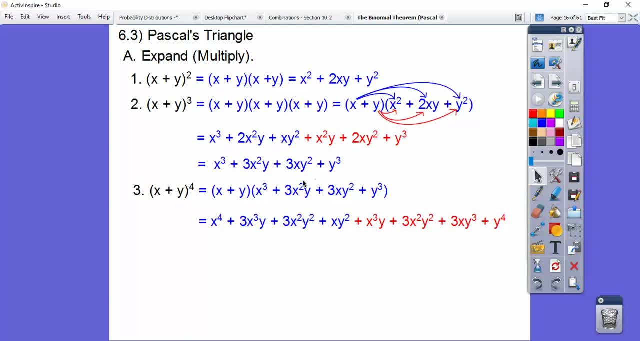 that is right there. And then combining the like terms: Okay, so we have an x cubed y. got another one somewhere here, right here, an x cubed. So there's four of them, because there's three over here And one right here. we have an x y. 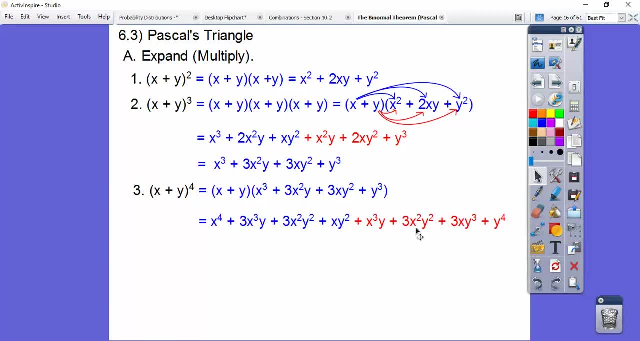 squared. we have another three of them right here, So there's four of those, Okay. there's no x squared y squared, So I'm sorry. there is two. three x squared- y squared. three x squared- y squared is six of those right there. So there's the answer right there, Okay. And now there is a reason why. 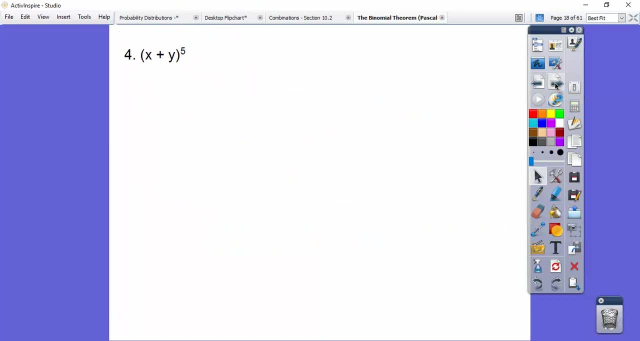 I'm doing this you guys. So if I asked you to do that, I'm not going to, you know, force you guys to go through that. I'm just going to show you the answer. Here's the answer, right there. So 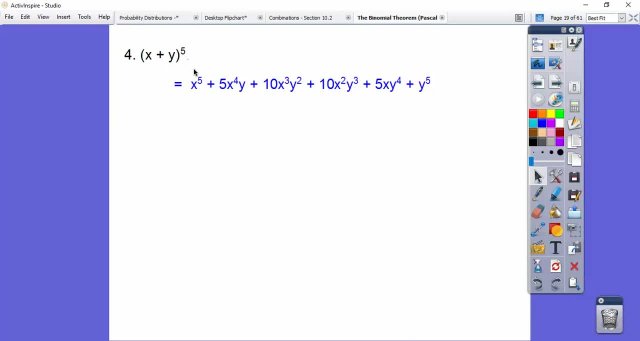 now how, whatever power that is, it starts with that power and it ends with that power. Okay, and then notice also the exponents they always add to this. this is five and this is four. this is one. four plus one is five, three plus two is five, two plus three is five And one plus. 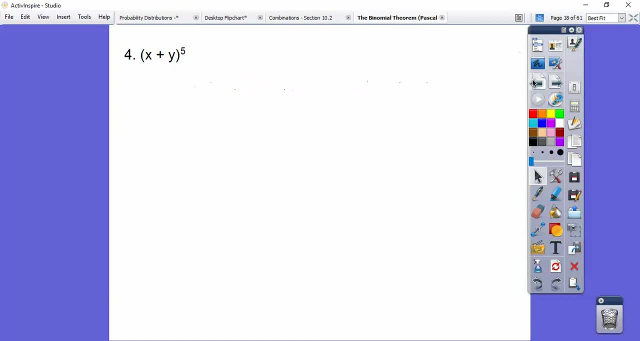 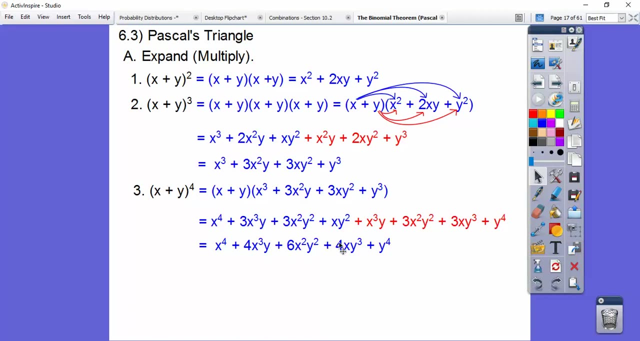 four is five, And so they're always adding. let's go to the fourth one right here. These always add to four. So here's a four. three plus one is four. two plus two is four. one plus three is four. They always add to four, This one, they always add to three, right there. 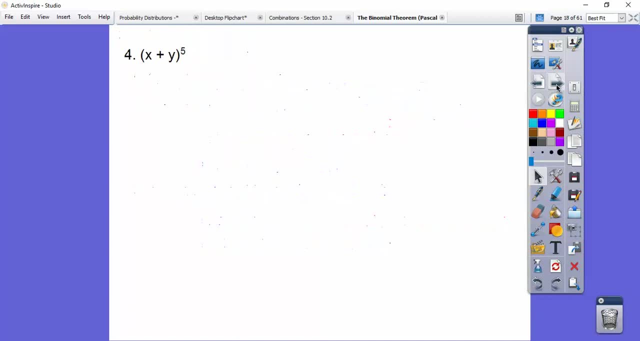 And then what I want you to see is: now let's go back to this one, This one's. they're all the same, you guys. So they go in d as one descends an exponent. So we have x to the fifth, x to the. 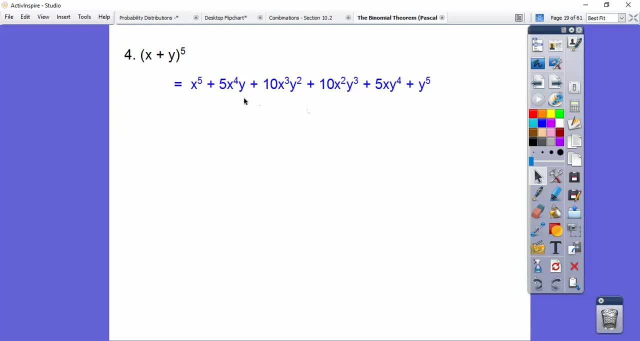 fourth x to the third x, squared x. As as x is descending, y is, they call it ascending, it's going up. So there's no y's here. We have one y, two y, three y, four y and then all five y's. 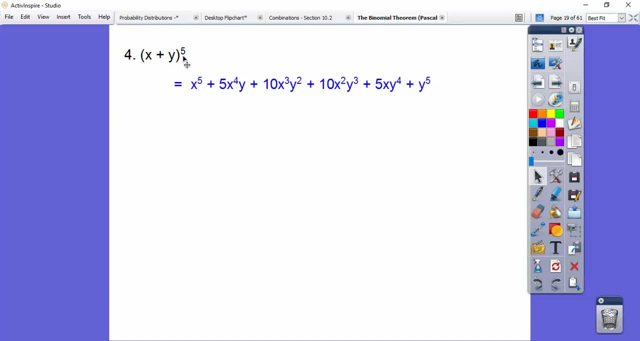 right there, Okay, So the exponents add to that and they descend with the first guy in there and they ascend, which means they go up with the second guy, And they always add to that. right there, the exponents. Okay, And I'll explain these numbers in front in just a second, That's. 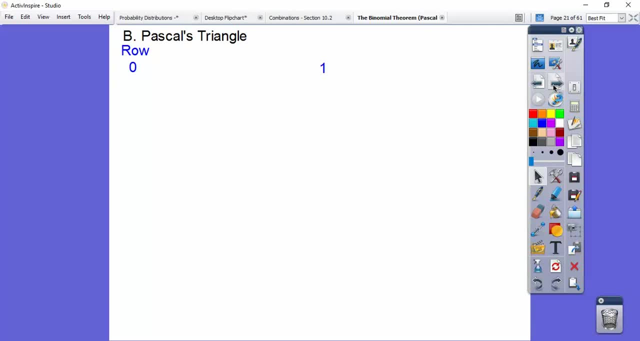 what Pascal's triangle is all about right here. So so Pascal's triangle. Now I'm going to do make sure you put this one right here, because we're going to make a big triangle going down like this. So it's make sure it's in the middle of the paper. 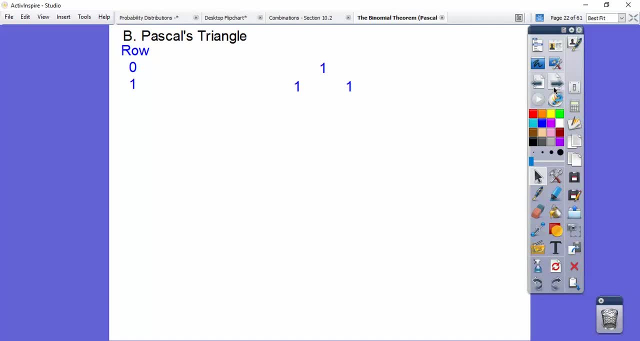 And this is row zero: Okay, Row one would give us this. Okay, And I know you don't see a pattern yet. Here's row two: Okay. Do you see a pattern yet? Probably not. Here's row three: Okay, Do. 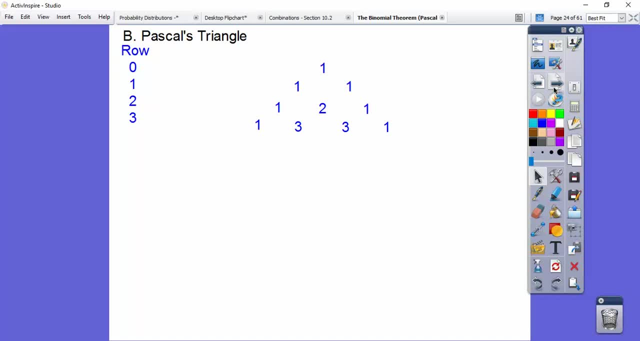 you see a pattern? yet That one? you might be able to see a pattern. How about this one right here? Do you? do you see a pattern right there? But the number here is the sum of the numbers on top. So one plus three is four. Three plus three is six. Three plus one is four. 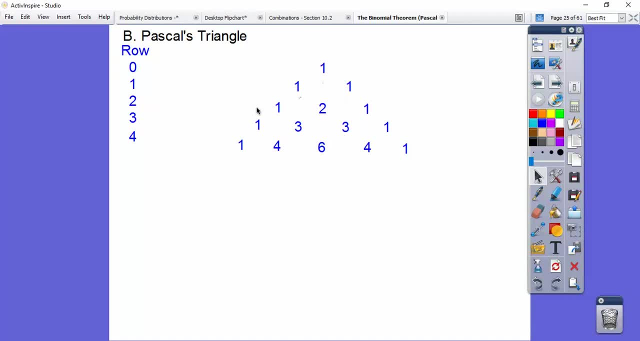 Okay, And then these are always going by ones down here. Okay, This three came from one plus two. This three came from two plus one. Okay, This two came from one plus one. Do you see that? So here we're going to start. it's going to be one, And then this number is going to be the sum of 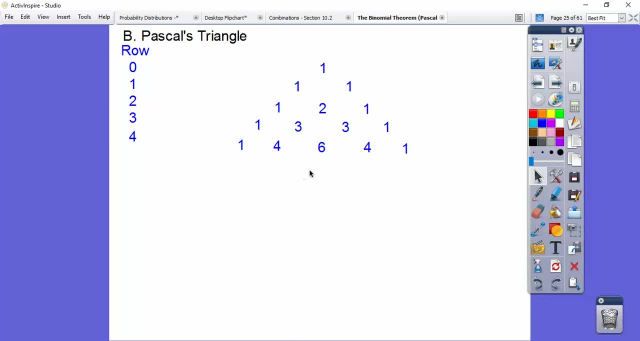 these guys, So five. sum of these guys 10, and then 10 again, and then five, and then one. Can you see? they're just the sum of the two numbers. So that's row five, Row six. we just keep adding. 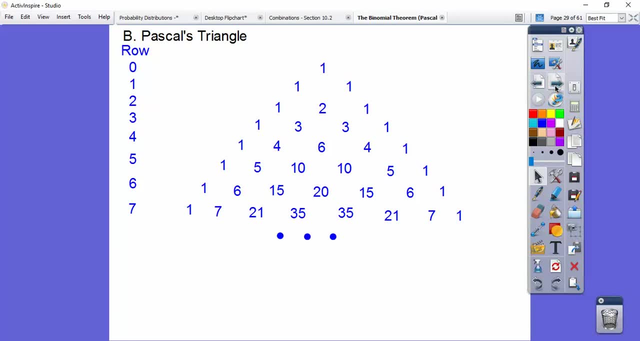 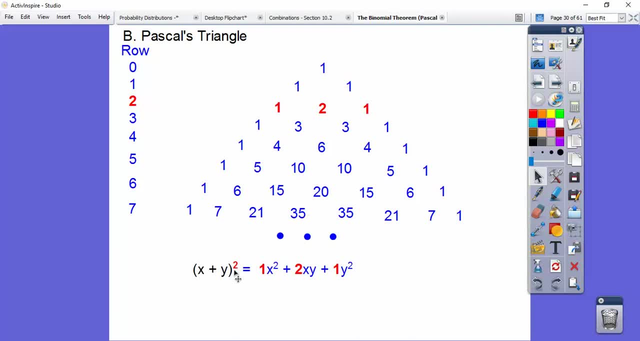 at the first one that we did When it was squared. when it was squared, these numbers here are the coefficients in Pascal's triangle for row two, row two, right there, Okay, And then remember the first one. it starts with all of the first one, So X to that power, right there, And then. 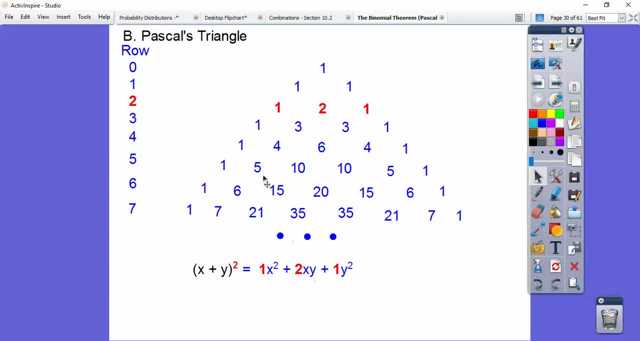 it goes down and the other one starts going up. Okay, And then these numbers. are these numbers right here? Okay, So look at this one. Here's X plus Y to the third power, If we go to row three: one, three, three, one. here they are: one, three, three, one, Okay. 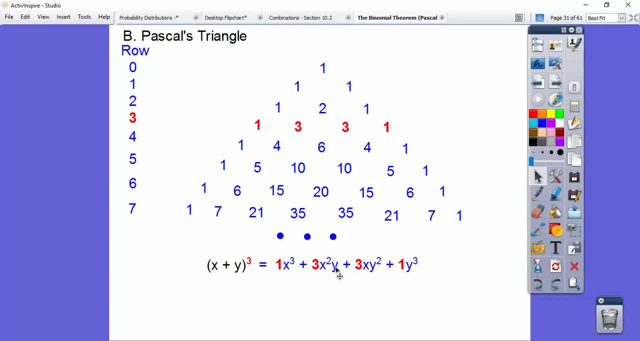 X to the third, and then it goes down and Y comes into the picture. X squared Y. And remember these exponents, add to this guy right there: X, Y squared. So we put those coefficients in there. And so here's the one to the fourth row: four one, four, six, four one. one, four, six, four one. 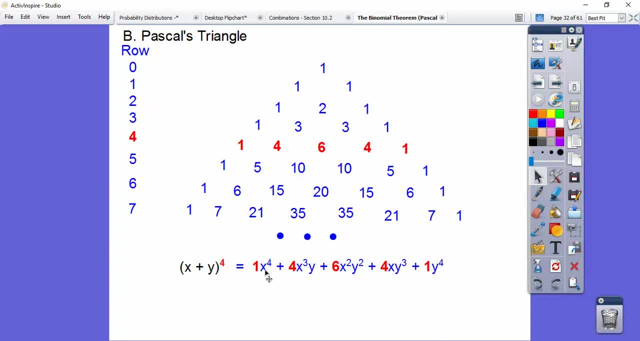 And the first one is X to the fourth, right there, And then we descend, So it's X to the third, And then Y starts ascending, growing up. So Y to the first, X squared, So X goes down, Y goes up. 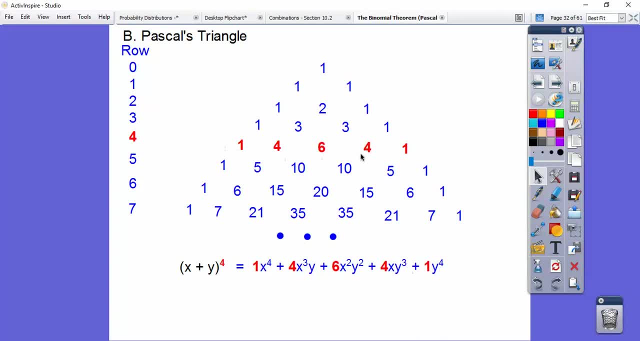 X goes down, Y goes up, And the red numbers are from row four And row four is from this guy. Row five would be X to the fourth, And then Y goes down, Y goes up, And then Y goes up And then Y goes up. 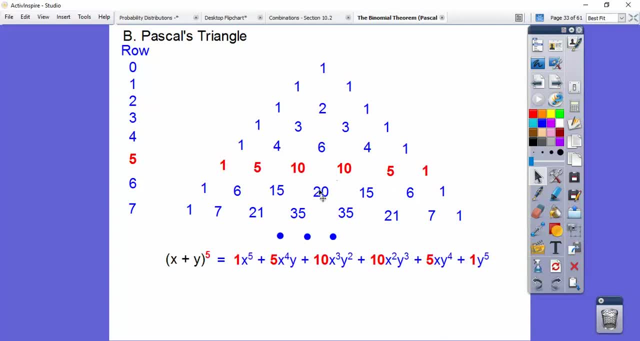 Okay, Row five is one. five: 10, 10, 5, 1, 1, 5, 10,, 10,, 5, 1.. Okay, X to the fifth, Okay, And then descend, ascend, So as X goes down, Y goes up, X goes down, Y goes up, X goes down, Y goes up. 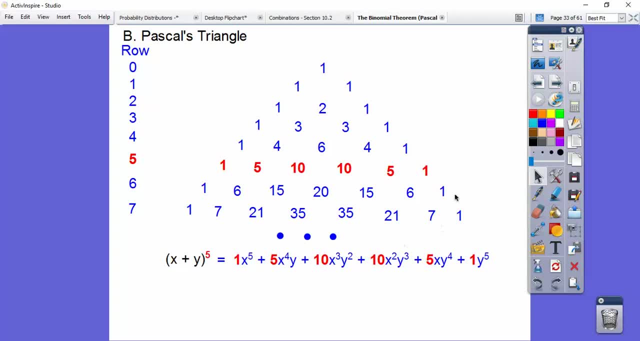 These powers add to this guy right there, Okay, And so on. If we did row six, it would look like this: Okay, One, six, 15,, 20,, 15,, 6,, 1.. There they are: X to the sixth, X to the fifth, Y. 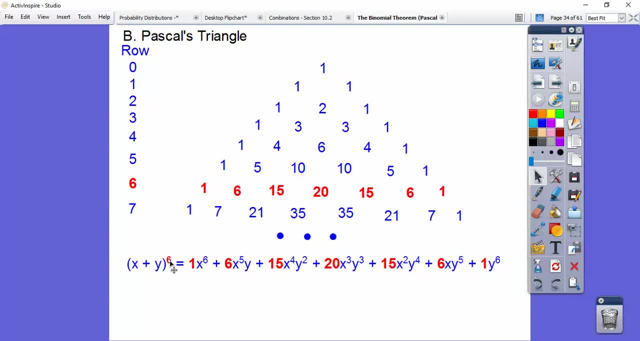 Remember these exponents always add to this guy, right here, Okay. X cubed, Y cubed, and so on, Okay. So, as X descends, Y ascends, right there, Okay. So let's use Pascal's triangle to expand this guy. 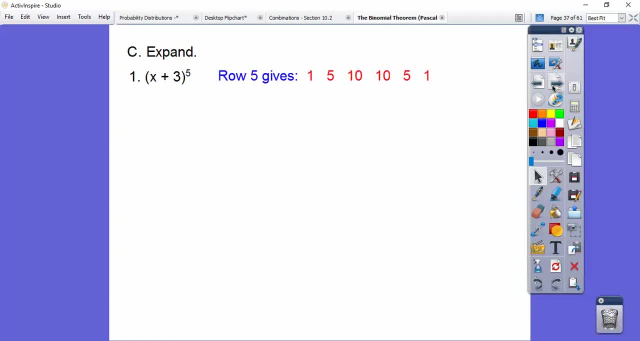 X plus three to the fifth. Okay, So we're going to go into row five right here. Now. this is our Y, right here. Okay, So row five gives these numbers. So it's going to be one. this guy to the fifth. 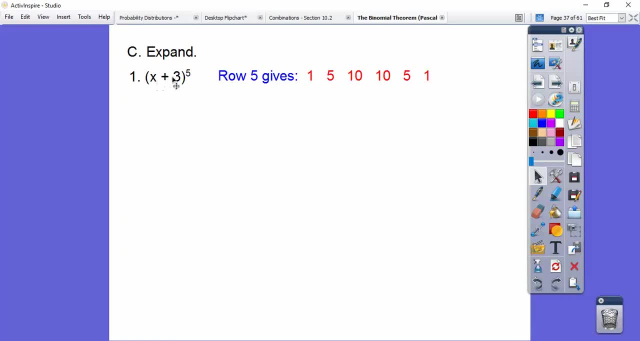 plus five, this guy to the fourth, and then three to the first plus 10.. This guy goes down, this one goes up, and so on. So here we go, Let's go ahead and put that in there. right there, Okay. 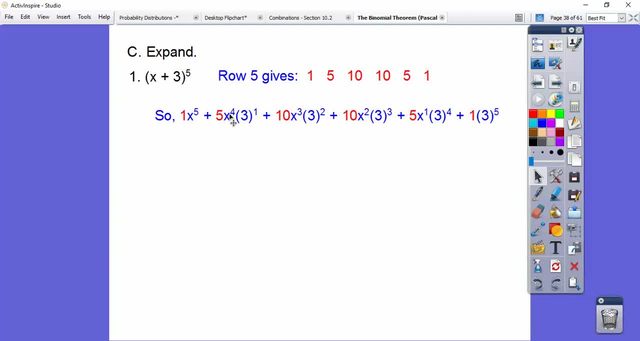 Notice how X goes down from five to four and then three comes into the picture, And notice how these exponents always add to that Five, right there, Okay, And we get these red numbers from Pascal's triangle in row five. Remember it starts with row zero. Okay, Row zero. 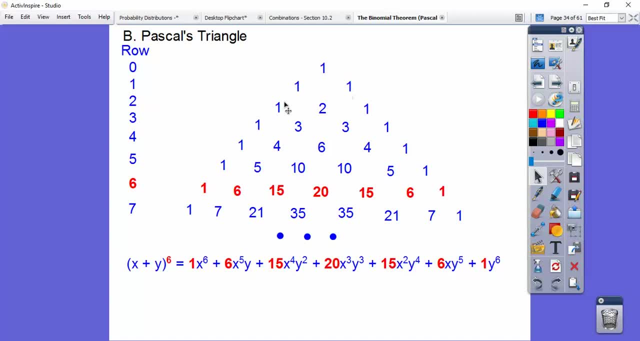 is one and row one is one and one. Okay, And then you can start your patterns for Pascal's triangle. Okay, So here we are, And then we got to go ahead and multiply here, So we got to do the exponents first. Okay, Three to the first is three. Three times five is 15.. Three squared is: 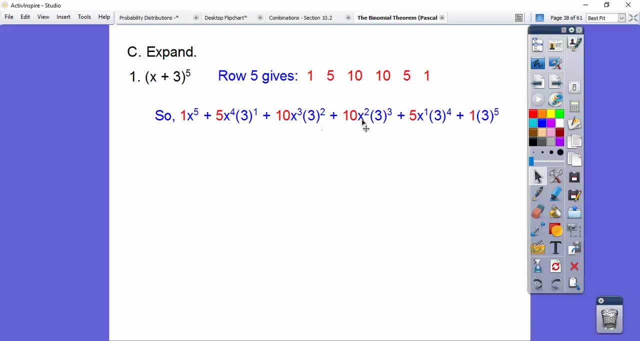 nine Nine times 10 is 90.. Okay, Three to the third is 27.. 27 times 10 is 270.. Three to the fourth is 81.. 81 times five is 40. And then we got to go ahead and multiply here, So we got to do. 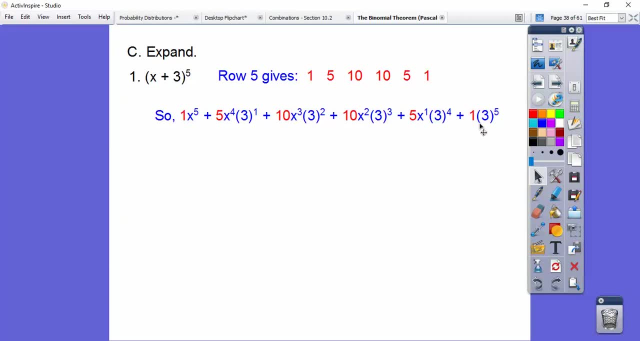 those exponents first, And then we multiply the coefficients together. Okay, So we get that right there. Okay, All right. So let's try another one here. you guys, I got a handful of them, So here's A plus 2B to the fourth. Okay, So let's go to row four. one, four, six, four, one, Okay, And then. 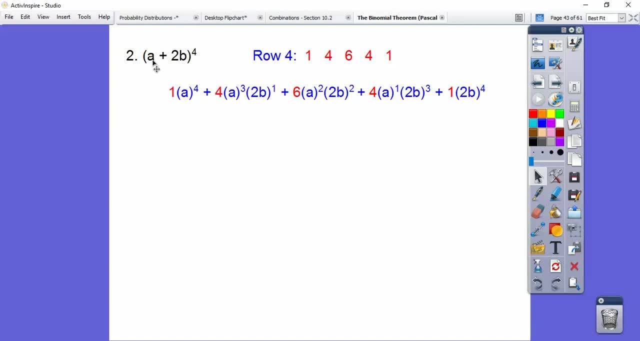 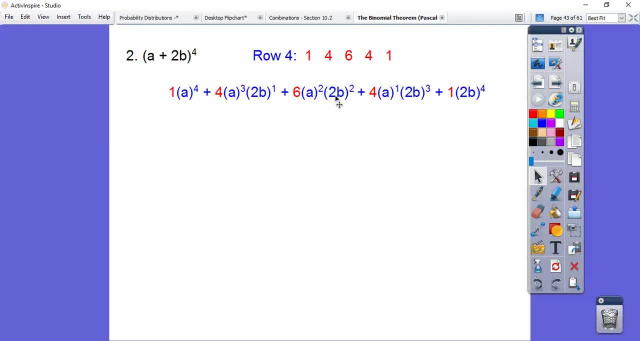 increases. Okay, Decrease A And the 2B increases. Decrease A And 2B increases. Okay, All right. So now we got to do two to the first B to the first. Here we got to do two to the second B to the. 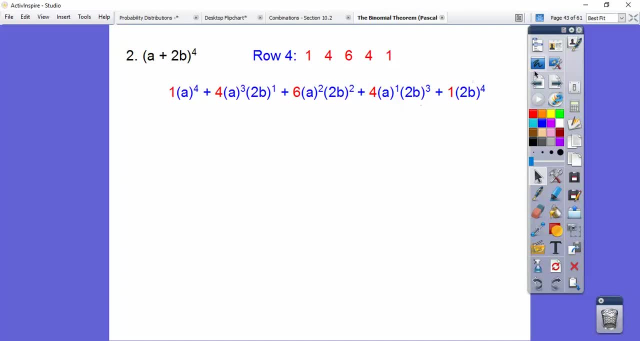 second: Okay To that power. Here's two to the third. B to the third, Okay. So that's going to get us that right there. Okay, Here's 2B to the first. Here's 2B squared. 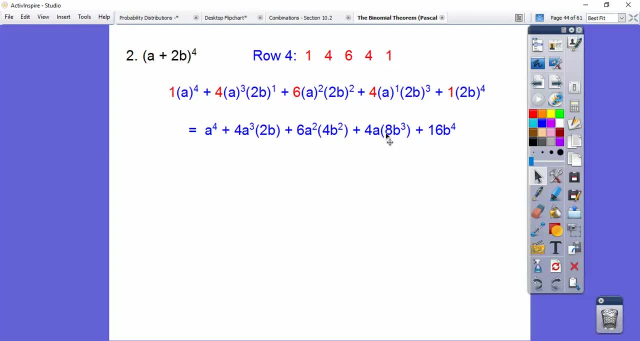 So 2 squared is 4.. B squared, 2 cubed, is 8.. And then B cubed, Okay, All right. And then we got to multiply the numbers here. So 4 times 2 is 8.. 6 times 4 is 24.. This is going to get us 32.. And 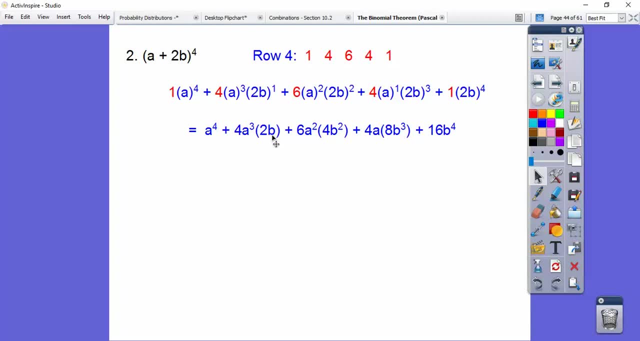 then we have A to the fourth. This guy's going to be A cubed B. This will be A squared, B squared, A, B cubed, and so on. So there's our answer right there. All right, Let's try one with the minus. 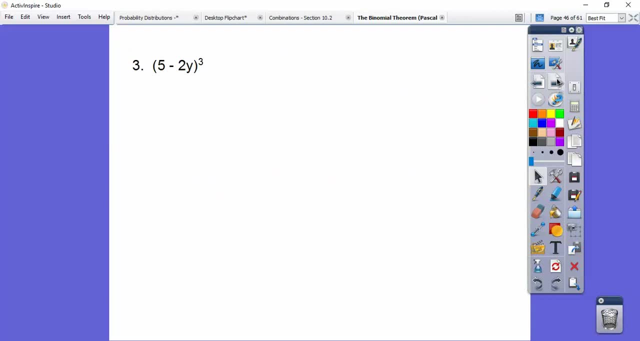 sign here. Okay, All right. So row three gives us those numbers right there. So let's go ahead and 1, 3,, 3, 1.. So it's going to be 1 times 5 to the third plus 3.. And then 5. 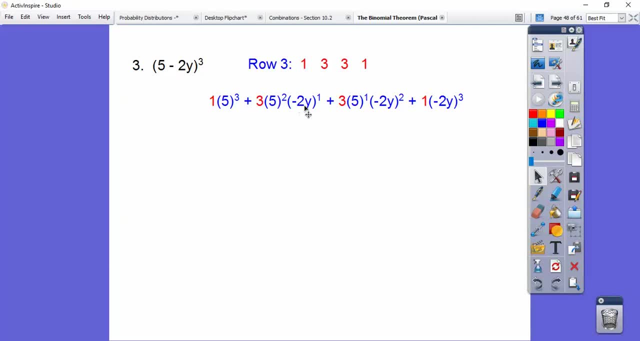 decreases And it's negative 2Y. So be careful: Negative 2Y increases plus 3. 5 decreases One exponent And then negative 2Y increases. Okay Now, the other thing we've got to remember is a. 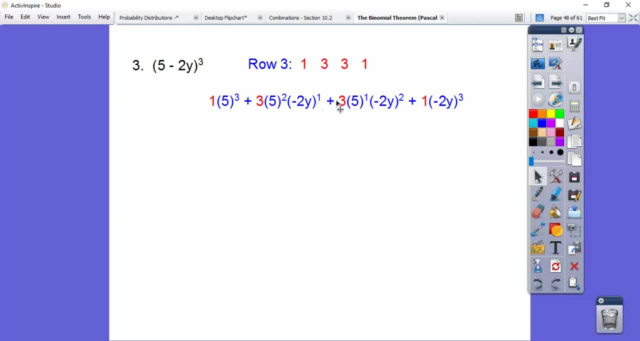 negative to an odd power is negative, Okay. So this is going to be a negative to an even power. So this is going to be negative. 2Y. This is going to be a positive 4Y. This is going to be a negative. 8Y cubed. Okay, 4Y squared. Did I say 4Y Anyway? so there's that. 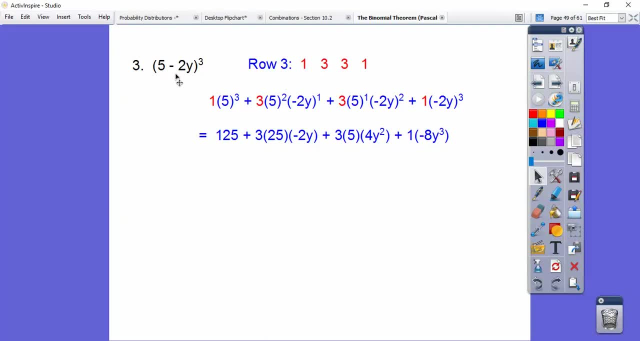 right there. Okay, So it's alternating signs. when you have a minus sign right here, It always alternates signs. So 5 to the third is 125.. And then 5 squared is 25.. Okay, I'm just doing the. 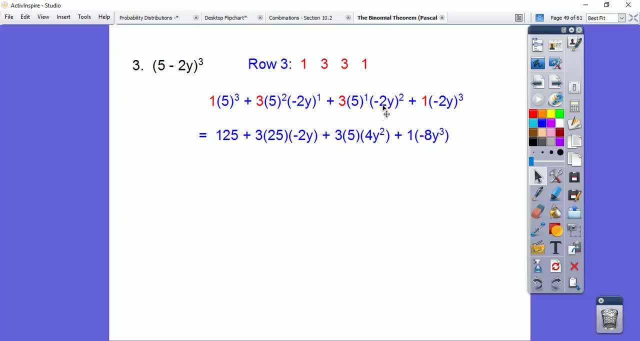 exponents here. Okay, So 5 to the first, And then negative: 2Y squared is positive, 4Y squared. And then negative: 2 cubed is negative, 8.. And Y cubed is Y cubed, All right, And then now we multiply, So this is going to be 3 times, 25 times negative 2.. 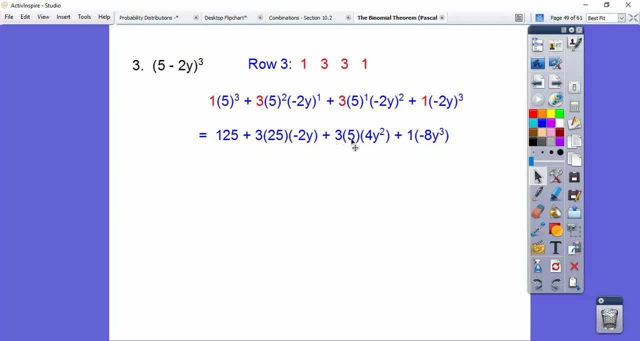 So what's that? Negative 150,? I think This is going to be 3 times 15, times 4.. So that's going to be a plus 60. And it's going to be a minus 8.. And then don't forget about your Ys on that, Okay. 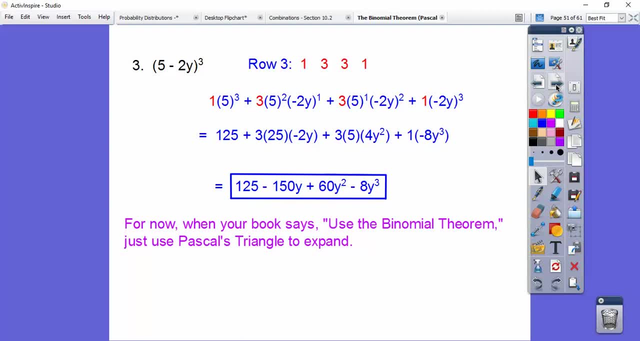 All right. So now your book is going to say: use the binomial theorem to expand. you guys Just use Pascal's triangle. for now We'll do binomial theorem stuff more. second semester- Okay, All right. So find the coefficient of X to the fourth and the expansion of 2X plus 5 to the. 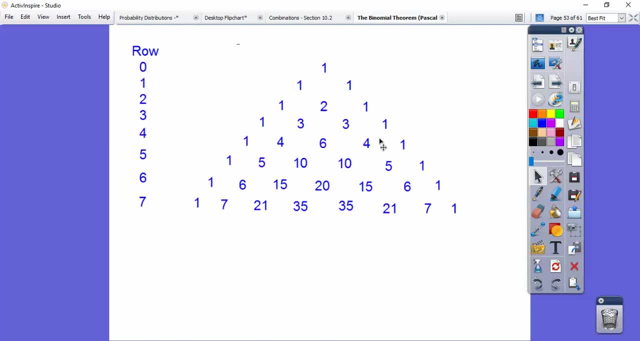 eighth. Okay, So we got to go. Here's the Pascal's triangle. We went down to row 7.. So row 8 is going to be 1, 8, 28.. What's that? 56,, 70,, 56, 28.. I'm just adding these numbers, 8 and 1.. So there's. 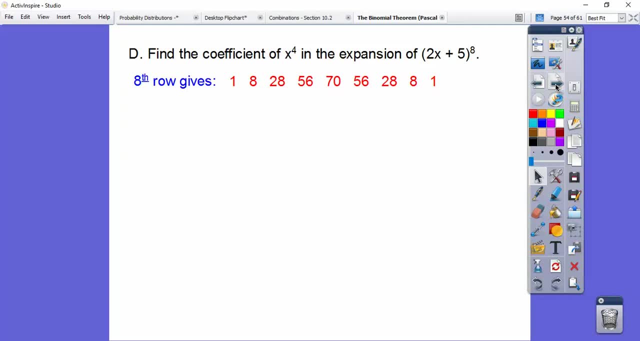 row 8, right there, Okay, And then those are the numbers. So it's going to be 1 with 2X to the 8. eighth, Okay. So this is asking the coefficient of X to the fourth. So this is going to be X to. 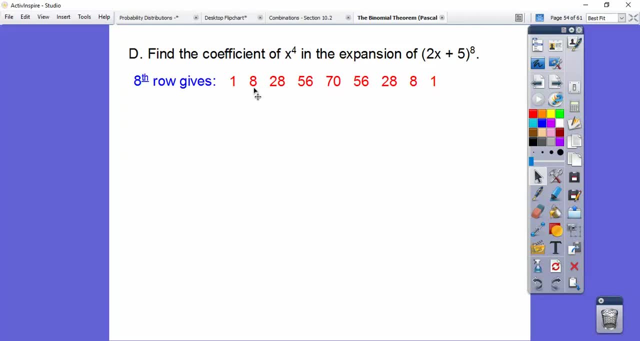 the eighth. This is going to be X to the seventh. This is going to be X to the sixth. This is going to be X to the fifth. This will be X to the fourth. I need that number right there. Okay, So it's going to be 70 and it's going to be this to the fourth times. this to the fourth, right there. 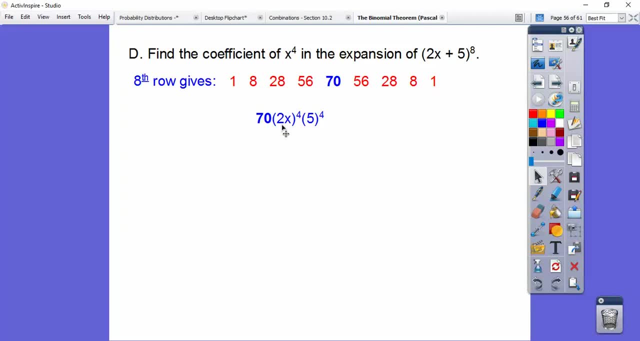 Okay, So. so there, it is right there. Okay, So there's going to get me my X to the fourth. Remember, this is this. this guy goes here: X to the eighth, and then this is going to be to the seventh, sixth, fifth, fourth, And it says: find the coefficient of X to the fourth. Okay, To the.